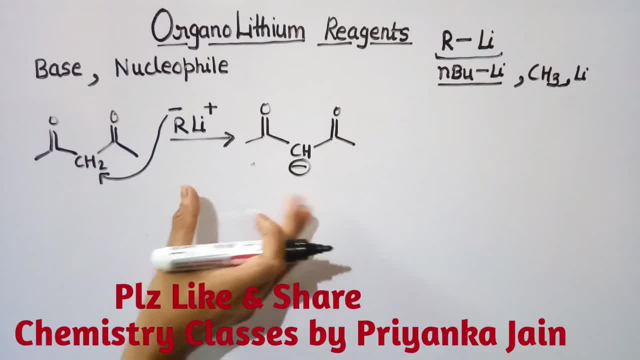 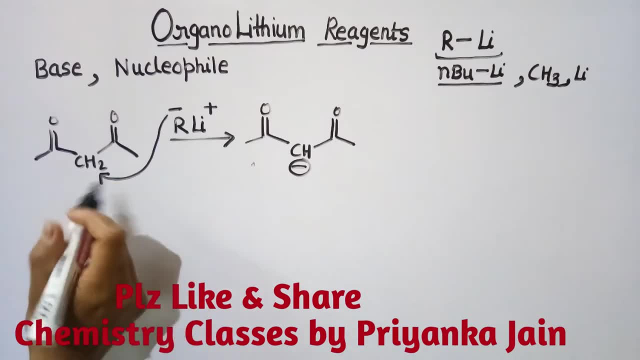 a new bond can be formed. Okay, So this is the proton abstraction reaction in the general. We will show you different examples of each type of the reaction. Firstly, see general reaction. Similarly, whenever it acts as a nucleophile, then what happens? 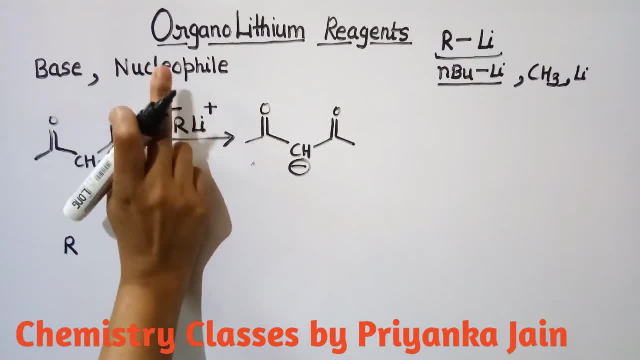 It can. When it is acting as a nucleophile, then it will add to the electrophile. Okay, So, for example, we know this is any carbonyl compound And in this there is a polarization of this type. So here comes a negative charge And here comes a positive charge. Right, 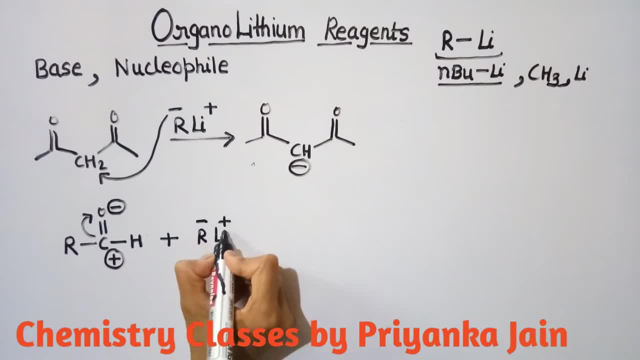 This will be negatively charged and this will be positively charged. Okay So this negative charge, this nucleophile, will attack here, at this electrophilic position. Okay, So a new bond is formed Here. a new bond is formed in this way. This will be R-Li Right And 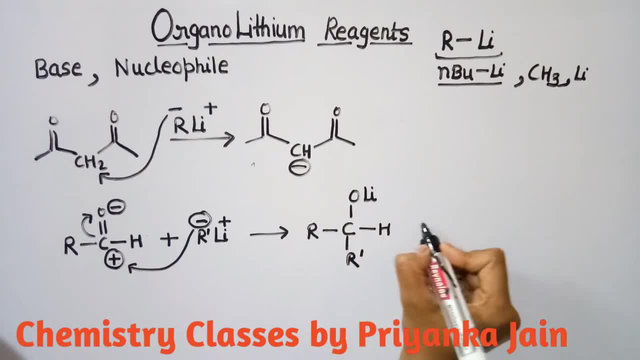 here the lithium will act And in the next step it will undergo the acid hydrolysis. So this lithium will get replaced by the hydrogen, so we will get this type of compound. I will show you different examples of each type of reaction later. firstly see this, okay. then see the another thing, how we can. 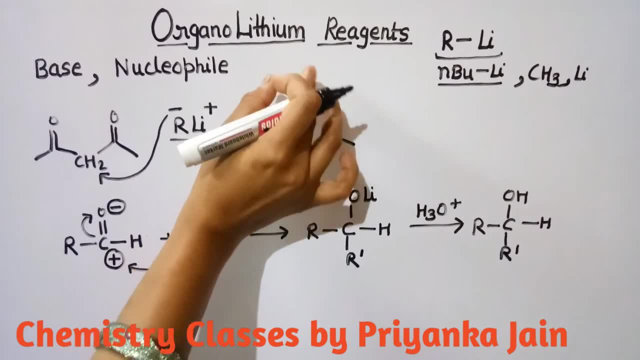 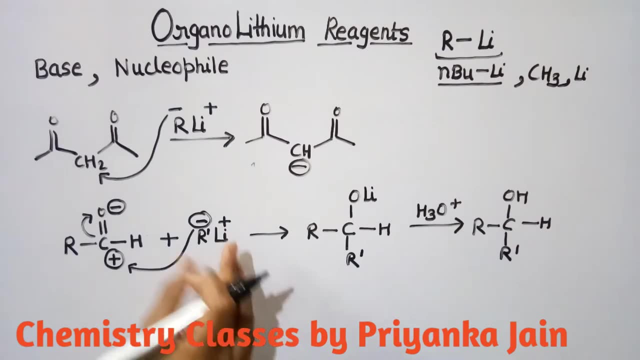 use the organo lithium reagents. these reasons are used in the ether solution at the low temperature, it means generally at the minus 78 degree centigrade by, because these are very good base so it can easily abstract the proton from the solvent. so in order to avoid the abstraction of proton from the 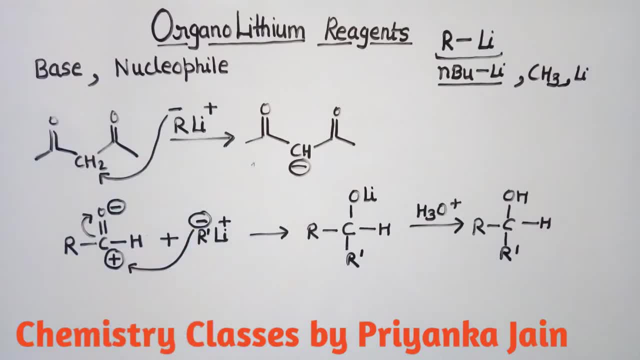 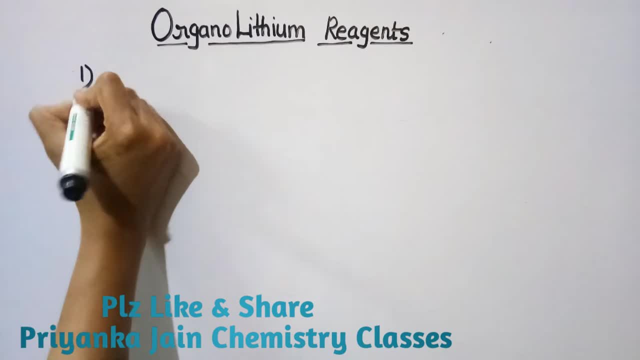 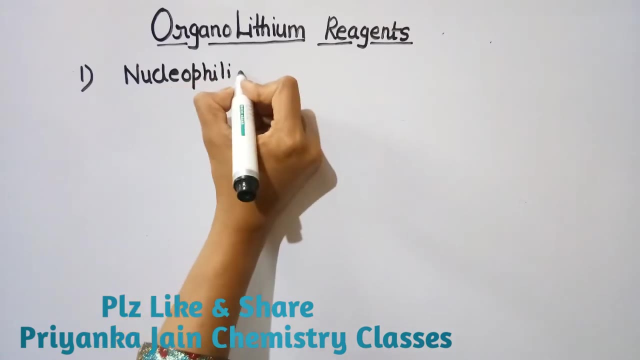 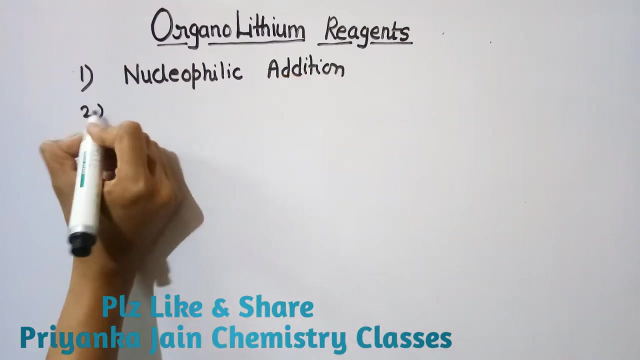 solvent. we will use them at the very low temperature. so in total, usually the organo lithium reagent shows five types of the reaction. first type of reaction is the nucleophilic addition reaction. second type is the proton extraction reaction when it is acting as a base. 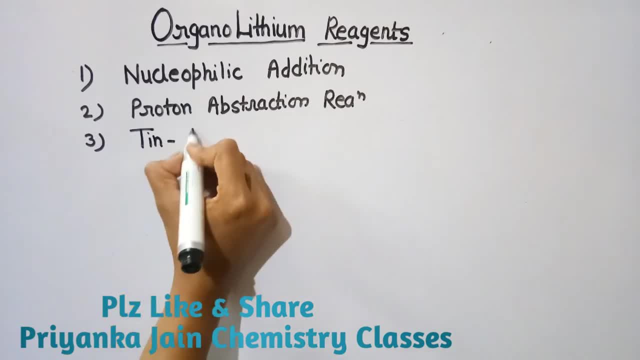 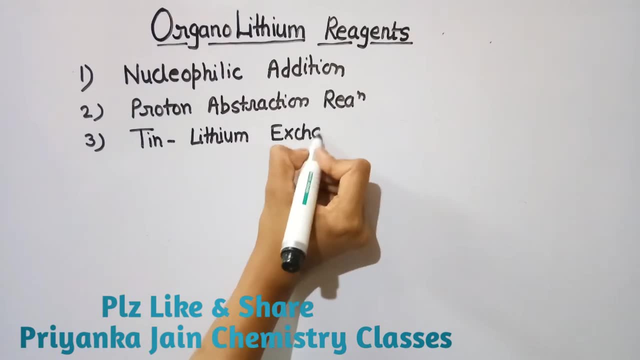 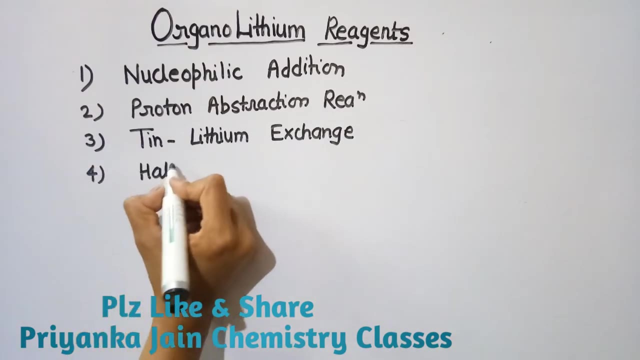 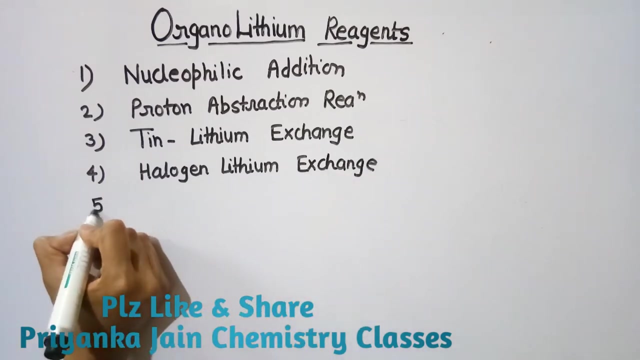 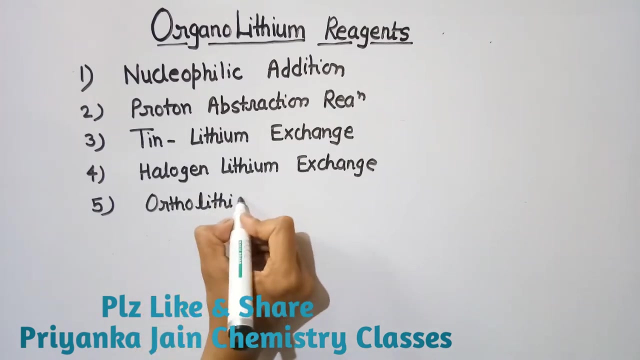 third one is the tin lithium exchange reaction. fourth type of reaction is the halogen lithium exchange reaction and the fifth one is the ortho lithiation. and now we have to see all of them one by one, with the help of the examples, along with the stereochemistry. okay, so firstly we see the nucleophilic. 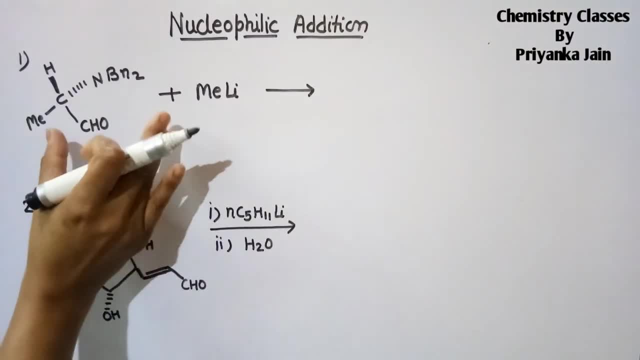 addition reaction. firstly, see here this is an example of addition to the carbonyl compound. here this is the carbonyl compound and when it adds to it, always remember this thing: that these reagents attack from the less hindered side. that side is free. here this group is present, this group is bulky, this is 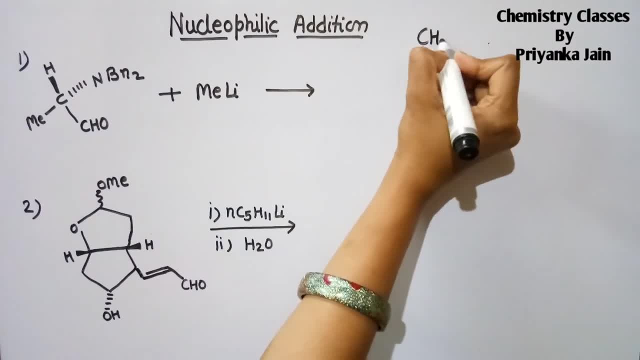 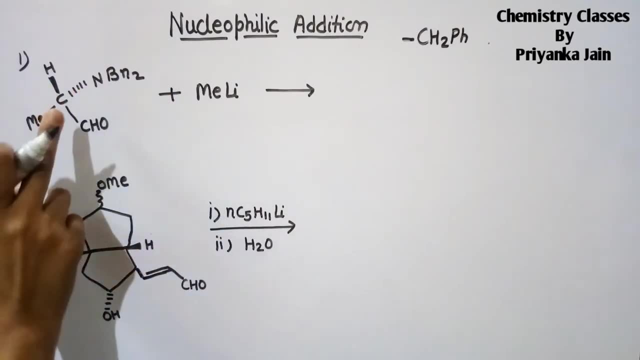 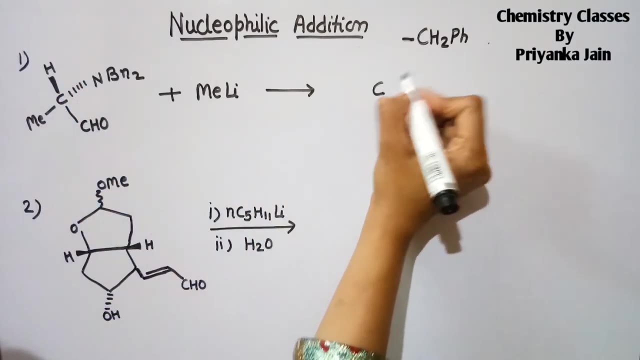 BN means this. BN means CH2PH group in this thing, so this is a bulky group, so the product will be such anti to this. this is below the plane, so it will be above the plane. the OH group will be above the plane, so this is below the plane. now we have to add that groups to. 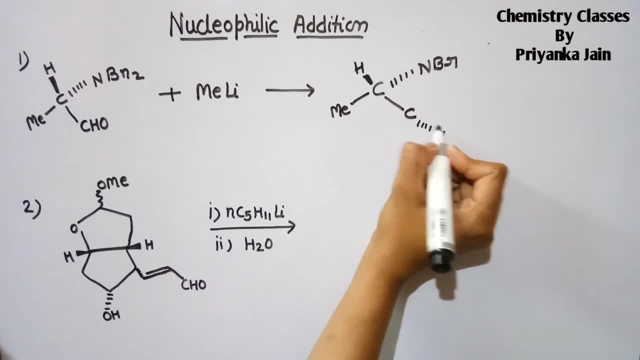 this. here one hydrogen is already present, right, and here the OH group will be added above the plane. Why? Because the reagent is attacking from the opposite side of this bulky group. So we are getting here the anti-product in this way. Okay. 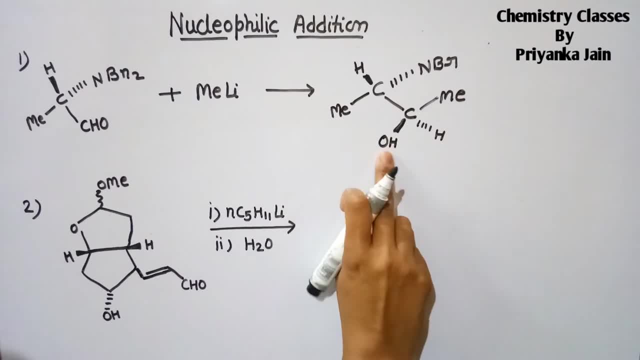 At one side the methyl group is added and this side O-Li group is added and by the acid hydrolysis is it? it is converted to the OH group Right Now. see the another example. This is the example of addition to the alpha beta unsaturated compounds, and here the addition will be always 1, 2 addition. 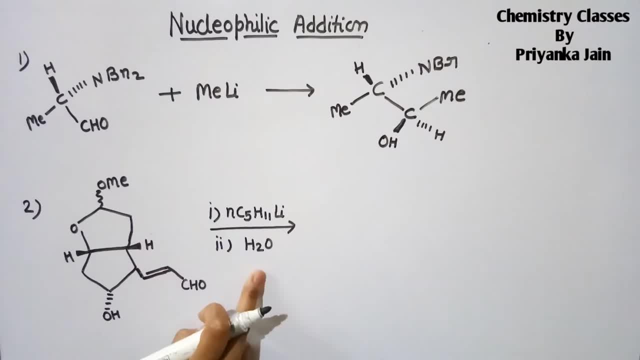 reaction. In the case of the Gilman reagent, I have told you, when you have seen the video of Gilman reagent, I have told you that their attack was 1, 4 addition reaction, but here the addition is 1, 2 addition reaction. Why? Because Gilman reagent was a soft nucleophile, while these all 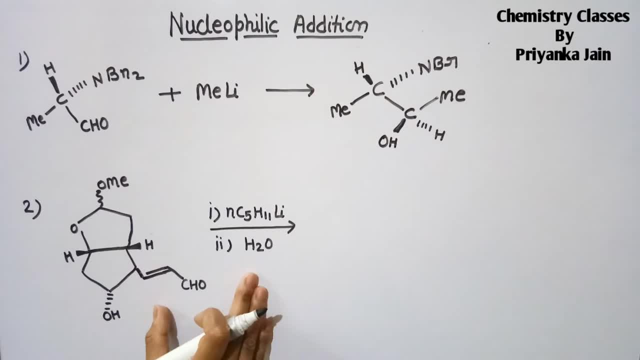 reagents. these organolithium reagents are hard nucleophile, So it will always attack at this carbon atom, particularly at this carbon atom. Okay, So the addition will be 1, 2 addition. Okay, So our product will be this all: 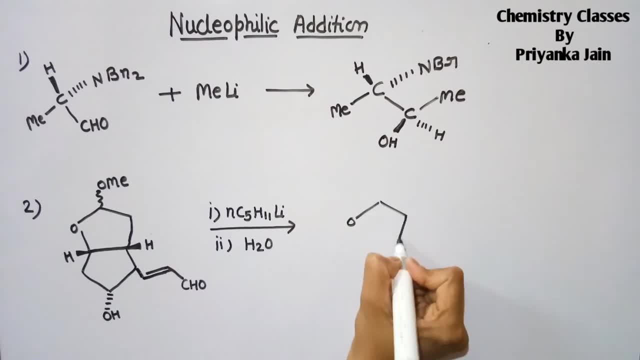 things of the this side will remain as it is because we have to add: at the carbon atom of the carbonyl group Now comes to this carbon atom, and here at this carbon atom one of the OH group is added Right, And at the other side we have to make the 5 carbon atom chain, because here we have given. 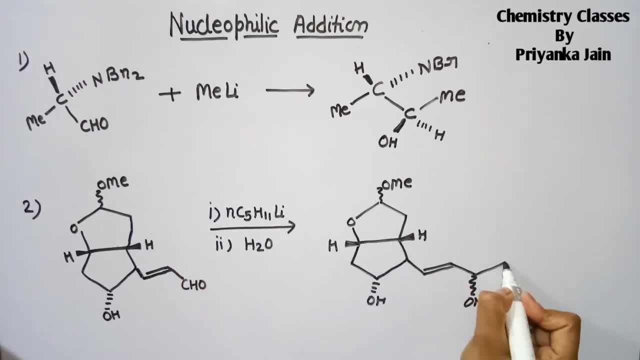 n-pentilithium. So now we have to make 5 carbon atoms: 1,, 2,, 3,, 4 and 5. In this way we are getting our product, Okay. Okay, Now see the another reaction: nucleophilic. 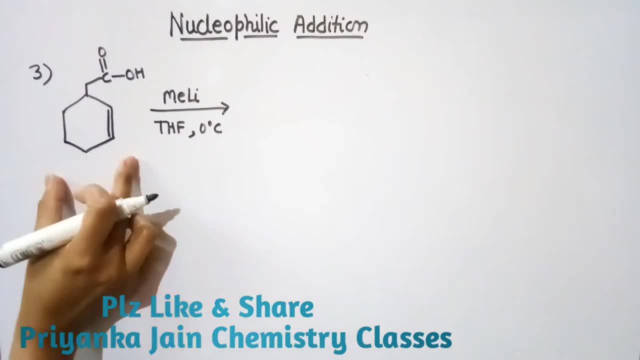 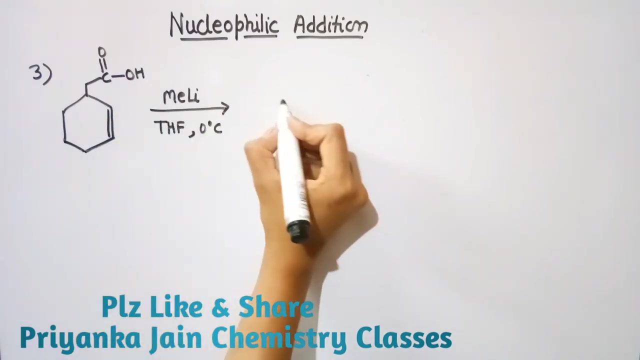 addition, reaction to the carboxylic acid When we have a compound with the carboxylic acid or a carboxylic acid derivative. In such cases we are getting the tertiary alcohol as the product. How We can see here. Firstly, this methyl lithium will add here. So 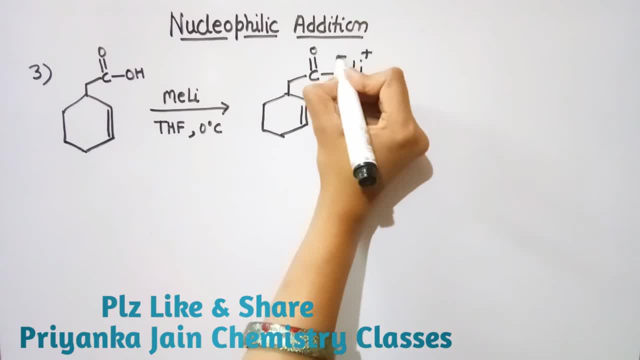 in this way. this will be plus, this is minus. We are getting the product Now. again. it will react with the methyl lithium. Then we have to react it with the ME3 SICLA and then do the acid hydrolysis. 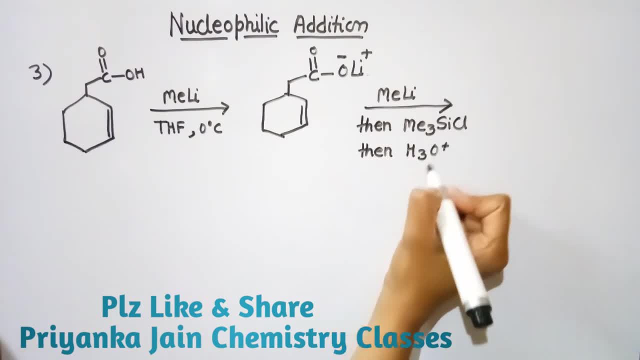 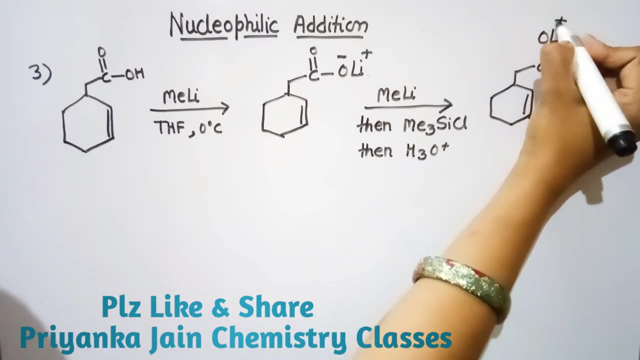 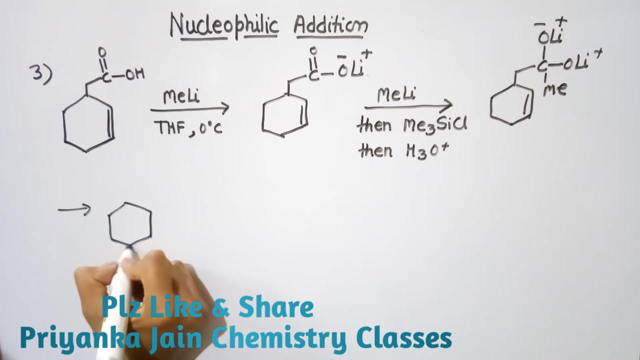 So what happens? Okay, Firstly, here another OLI plus group is attached. Okay, And here the methyl group. Now it will undergo the hydrolysis, So these both will convert to the OH groups, And this is methyl. Now we know. 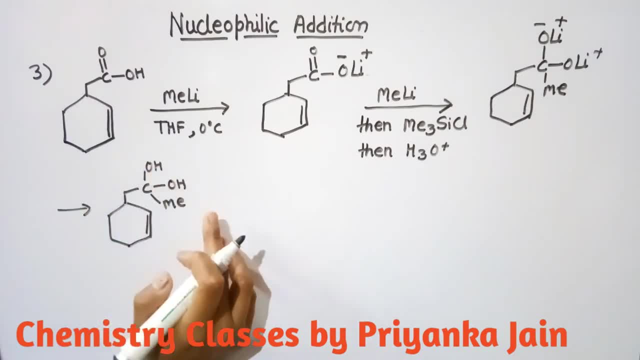 the same carbon atom, two OH groups cannot be happen, So it will undergo the decomposition. So here a carbonyl group is formed from here. in this way The water molecule is removed. Okay, So we will get this product, That is a ketone. 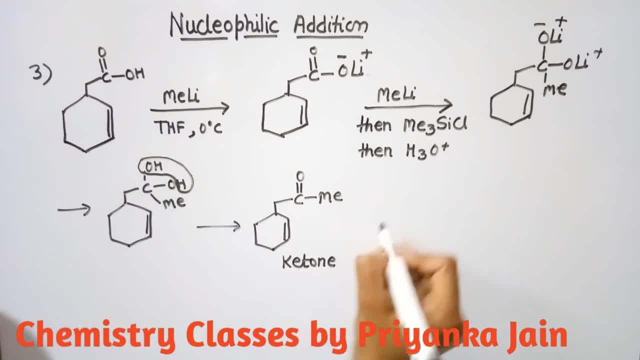 Okay, it can again react with the CH3 Li, so it will further undergo the 1- 2 addition reaction at this carbon. ok, so here again OH group is formed and methyl group is formed. so in this way we are getting the tertiary alcohol, next type of the 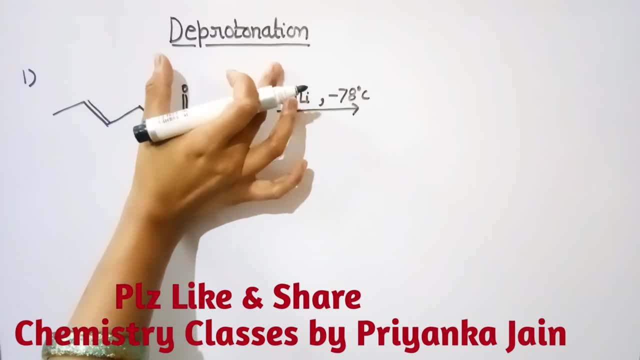 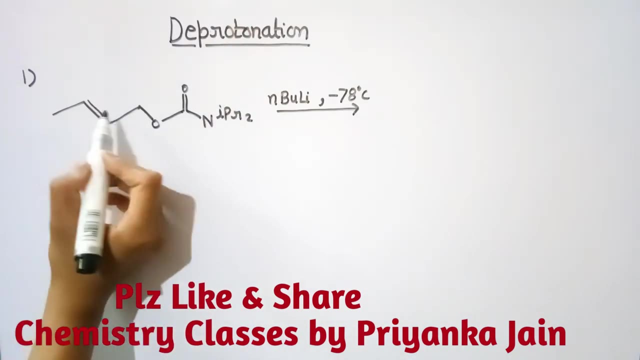 reaction is the deprotonation reaction or the proton abstraction reaction, as I have told you that these are the strong basis, so it can easily abstract the proton. it means the most acidic protons can be abstracted easily, for example here. here you can see this is the allylic position, so this proton, the 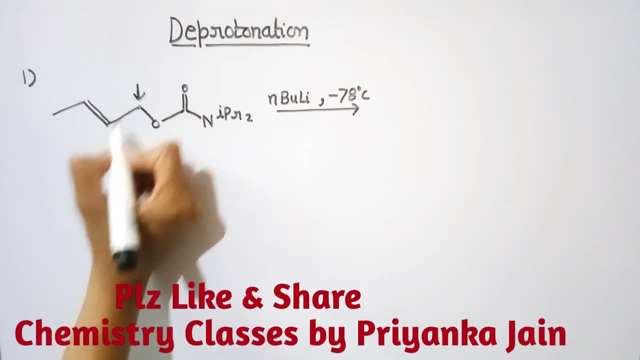 proton that is present at this position will be most acidic. whenever the allylic positions or the benzylic positions are present, then at this situation it can easily be abstracted. and it can easily be abstracted if it is position. the acidic protons are present and in this case particularly there is ortho carbonyl. 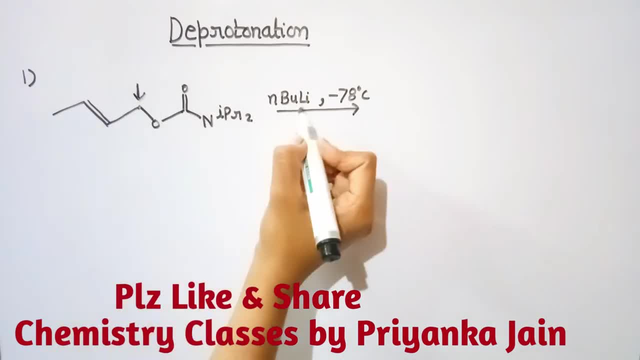 group present, so this becomes more acidic. so this can be easily abstracted by the lithium reagent. so this will abstract this proton. so as a result here we can represent it in this way- this will be minus charge and here will be positive charge. it means the proton has been abstracted. 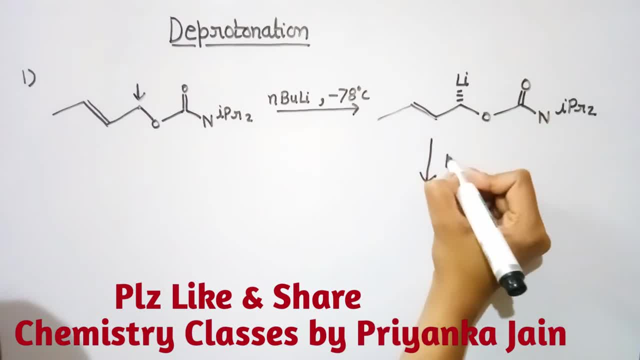 now, any electrophile can attack at this position and can form the bond. suppose we have this tributyl tin chloride. if we have this reason, then this can easily can form a bond. so this is the proton which we can easily extract from the more acidic position. 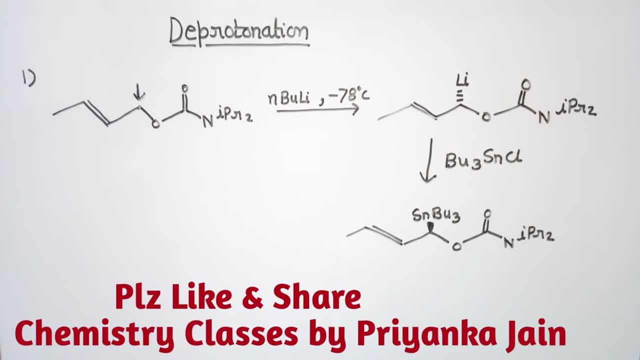 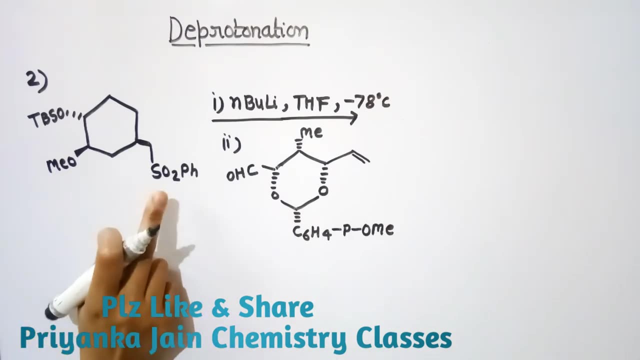 in this way so we can easily abstract a proton from the more acidic position and then we can treat it with the electrophile so we can form a new bond. now see this example. here i have taken a sulfoxide. when we treat sulfoxide with the n-butyl lithium, 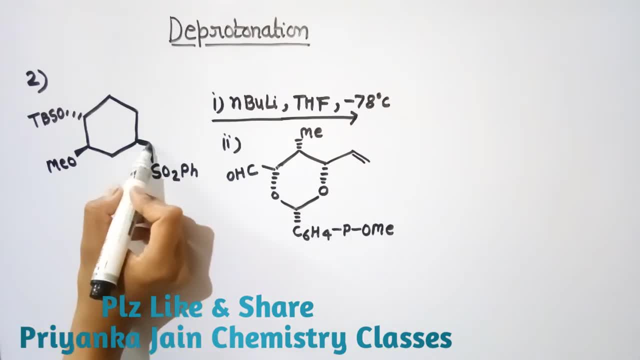 Here, in this case this hydrogen atom, at this carbon atom, the carbon atom that is alpha to this sulfur atom, At this carbon atom, the hydrogen will be most acidic, So this will be abstracted by the base, So it will abstract this proton. 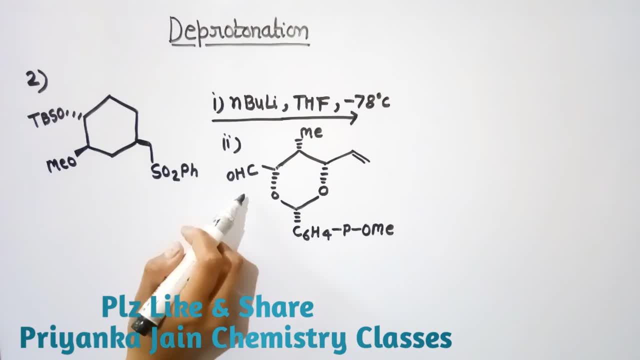 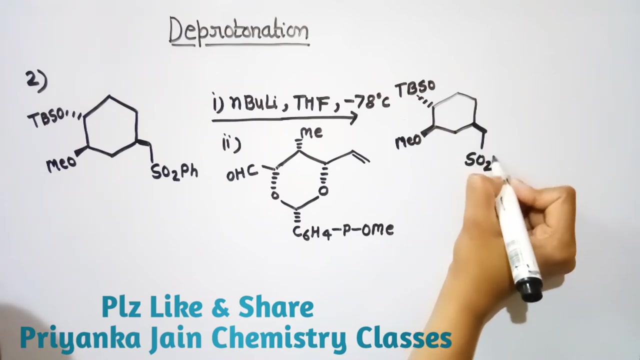 Then we are treating it with this compound, this carbonyl compound. So what happens here? A new bond is formed between this carbon atom, and this carbon atom Means to say: we can see, here this is our compound and here this is the group TBSO and this is the methoxide and this is the SO2PH. 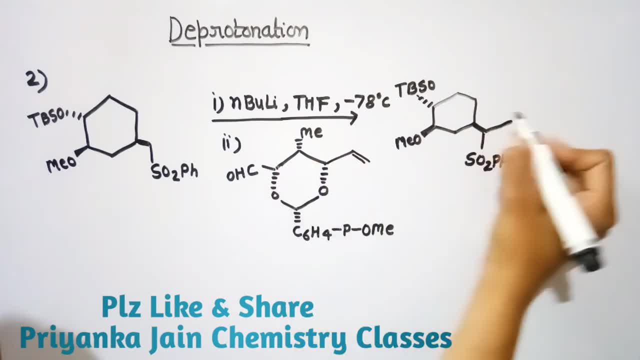 Now, at this position. this is the carbon atom of this. We can show it in this way And to this position. here will be the OH group. This wavy line means either it can be above the plane or below the plane in any manner. 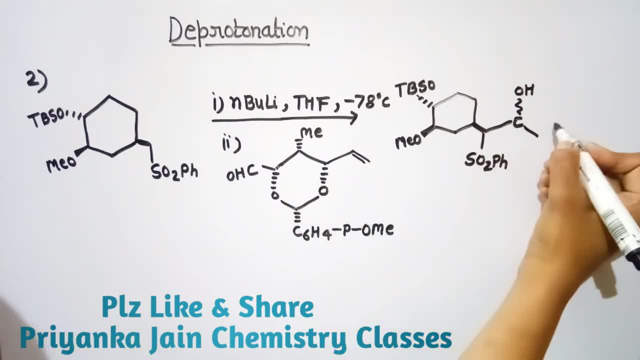 Right, And this is the rest of the group. We can show it in this way. So you can make this structure yourself In this way. this will be the whole structure. So we have to show here that there is a bond formation between this carbon atom and this carbon atom. 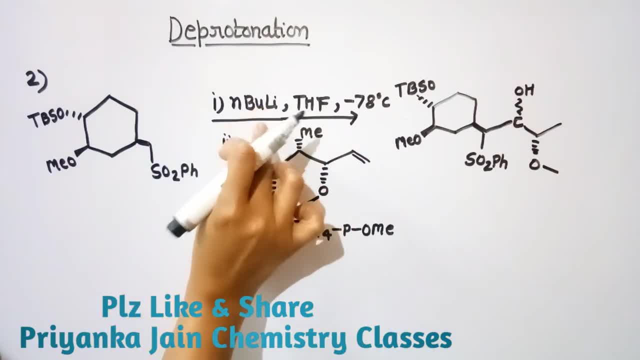 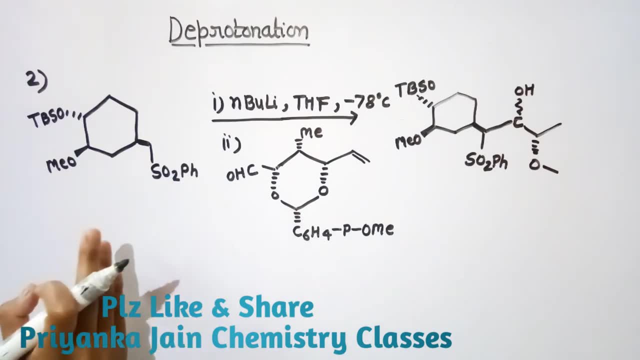 So this is the aim of the goal of this reagent: to abstract the proton from this position and form the bond between the electrophile and this carbon atom Right Now- see the case of the 1,3-dithions. 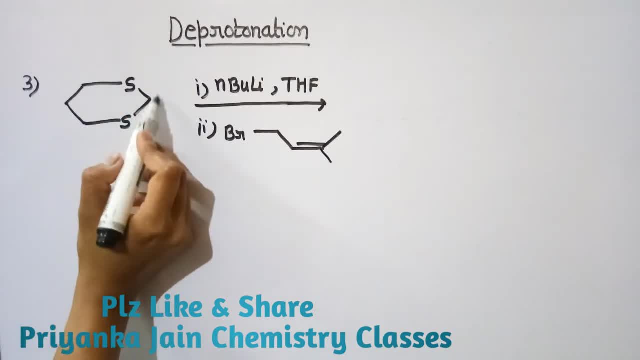 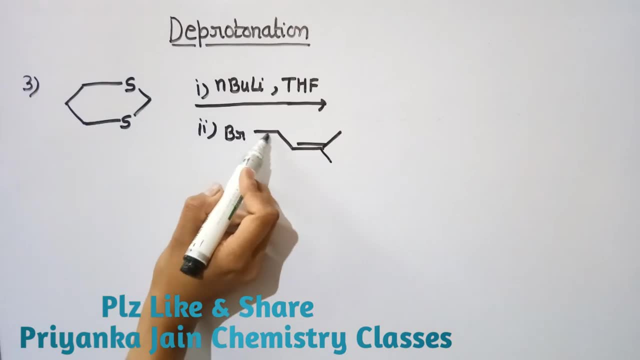 In this case, the proton will be abstracted from this position. This is the most acidic position, So proton will be abstracted from here. Now this position can form a bond between, with this carbon atom Right, So mean to say: 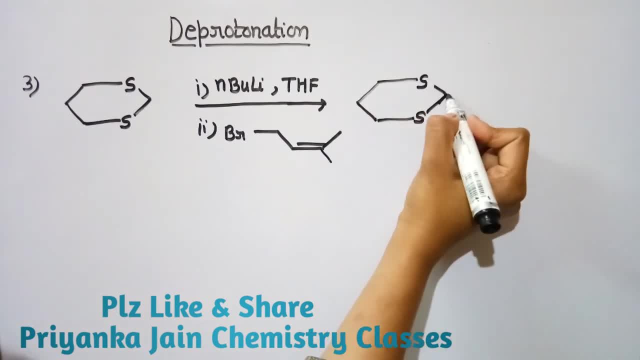 firstly, a proton is exacted from this position and then a new bond is formed with this carbon atom. So we are getting a new carbon-carbon bond. And then what is the purpose of these 1,3-dions? These are used for forming new compounds. 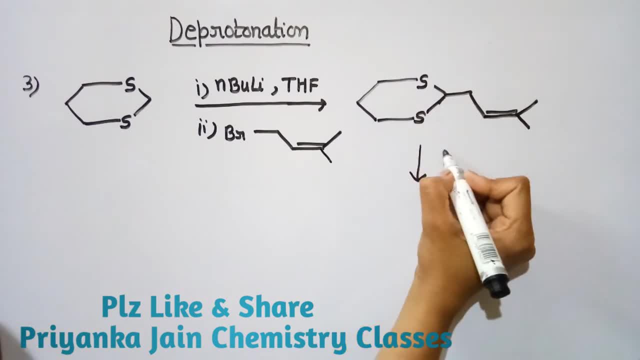 And here we can hydrolyze them to get the carbonyl group. So hydrolysis is here done with the mercury And we can do the co-cure science in the presence of S3O+. So this group will convert to CHO group. 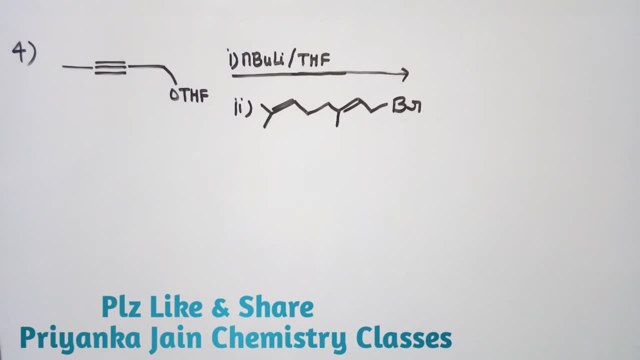 And we get this compound. Now see the another example of the proton abstraction from the terminal alkynes. In the case of terminal alkynes, this carbon atom is the most acidic, So the proton will be abstracted from this position. so when we abstract the proton from this position and and react it with the 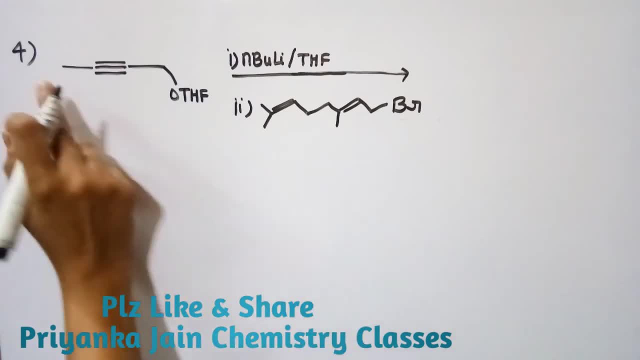 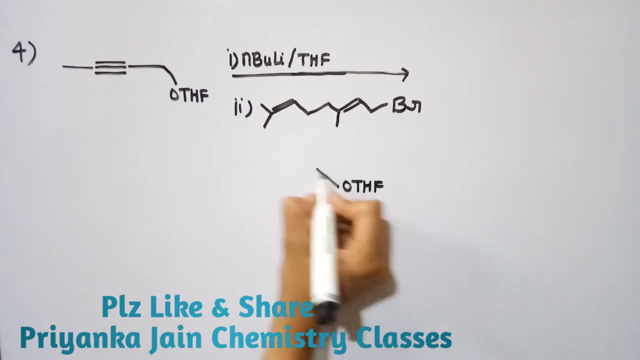 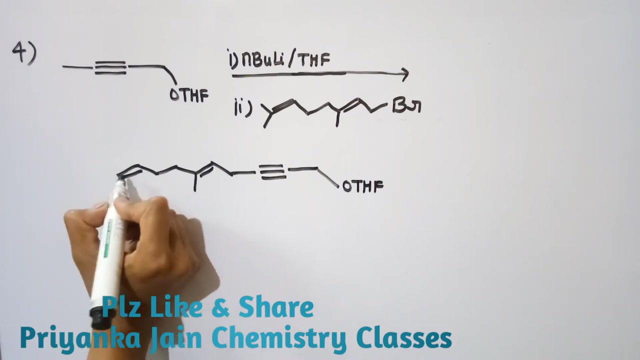 another compound like this. what will happen? a new bond is created between this and this position. so this is our carbon atom and now we have to form bond here. this is carbon atom and this is the new bond formation. rest of the compound remains as it is, only we have to just see this bond. 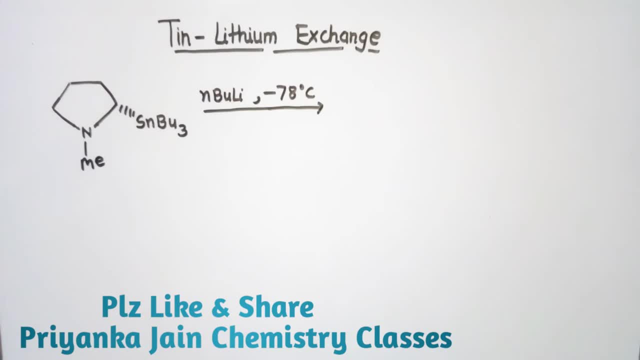 formation. next important re: Freiона elle Rainer. in lithium exchange reaction s from the name you can understand. if there is tin transp litigation present in atom is present in the compound, then it can be easily replaced by the lithium atom. the exchange of the tin by the lithium in the presence of 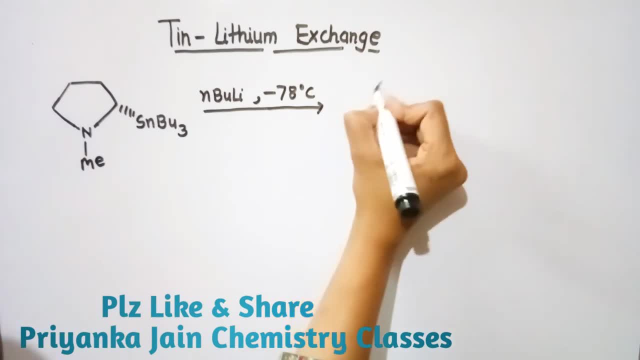 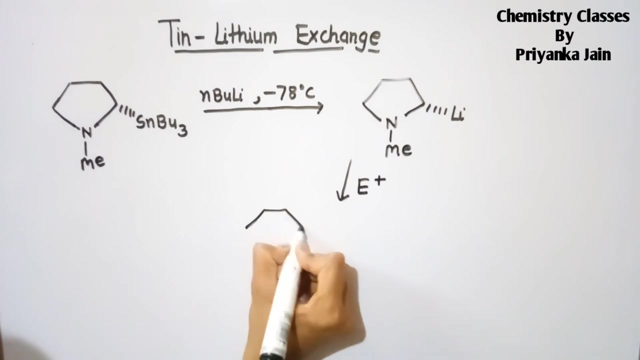 the organo lithium reagents. it means this compound is now converted in this way: this has been replaced by the lithium and now we can treat it with the any of the electrophile. we can react it with any electrophile. so that what will happen? this lithium will get exchanged by the electrophile. 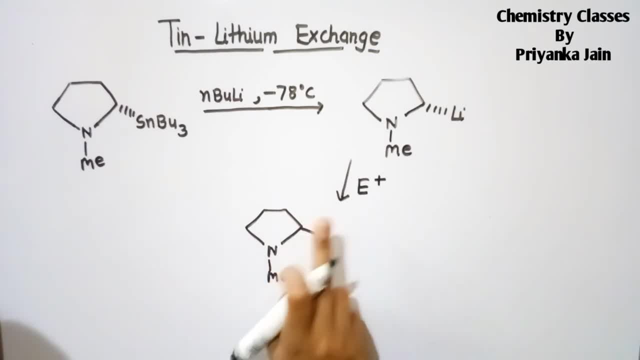 so here we will get the electrophile. now see, here, this is below the plane, so it will also be below the plane. okay, in this way, right? so the motive of this reaction is to provide a root for the synthesis of alpha hetero atom substituted organo lithium reagent. here you can see, this is the nitrogen atom. so 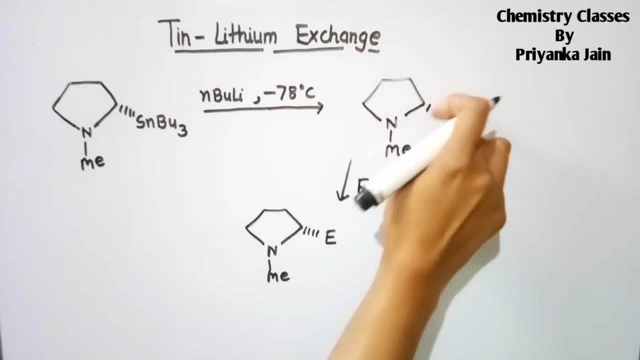 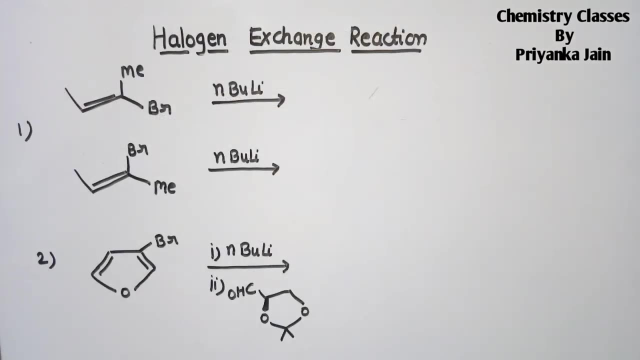 hetero atom is present and we can substitute a lithium atom at this position and then we can replace it by any of the electrophile and we can form a new bond here at the or two position of this nitrogen in this hetero atom. ok, now see that I know that important reaction that is halogen exchange. 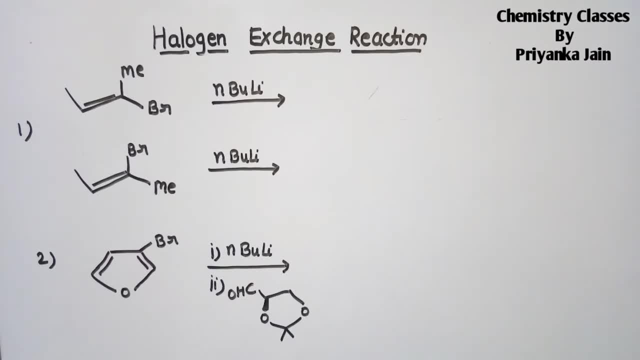 reaction similar to the lithium exchange in exchange reaction till lithium-ion exchange reaction is also significant for the hydrogen reagent exchange reaction. this is similar to that. here the replacement is of the halogen by the lithium and these reactions are highly stereo specific. it means the stereochemistry will remain as it. 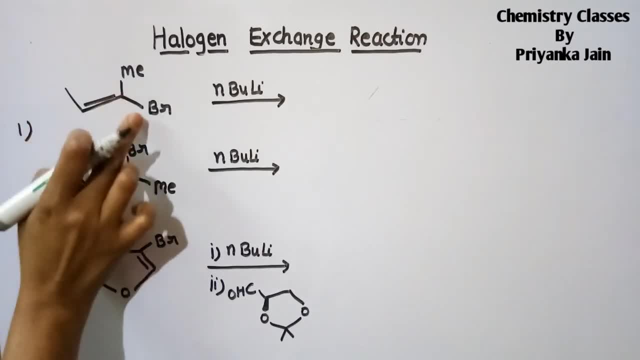 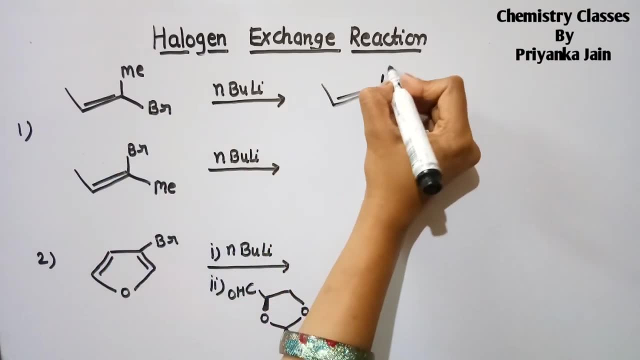 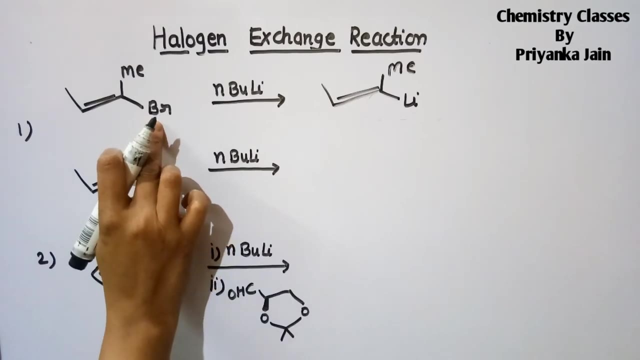 is as that in the reactant, for example, here in this case, this bromine is present here, so just we have to replace this by the lithium. it means the exchange of the halogen by the lithium, simply, and the stereochemistry remains as it is. similarly here: 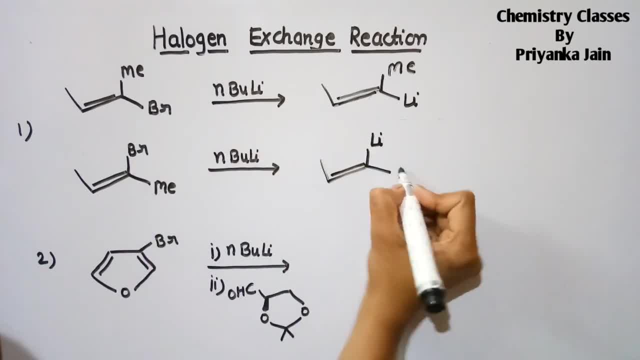 this is here, so the lithium will be here, okay. it means the reactions are highly stereo specific. now see this example. in this example, halogen is present here, so the abstraction of the halogen will take place from here. so this will now convert to the lithium. okay, and in the next step we are treating it with the. 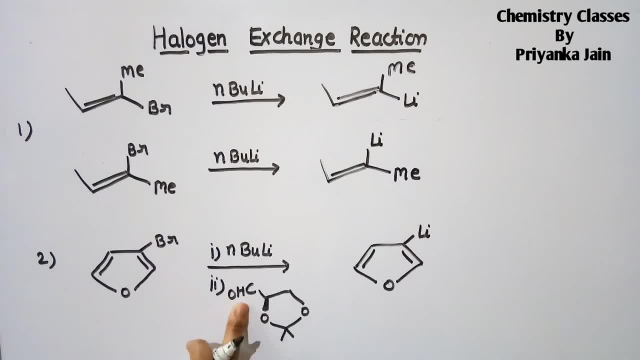 this compound, the electrophile. so what happens? a new bond is formed between this carbon atom and this lithium. so we have to form here a new bond now in this way, and the rest of the things remains as it is the same. and this is the reaction here. 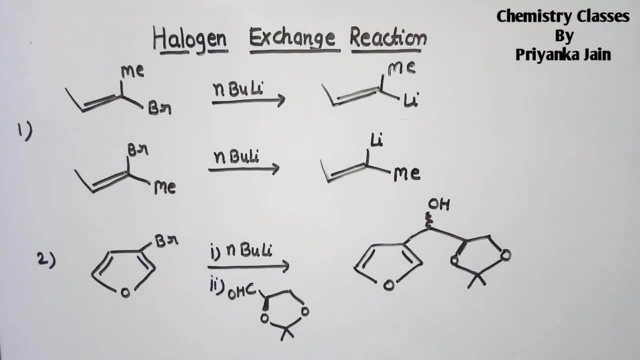 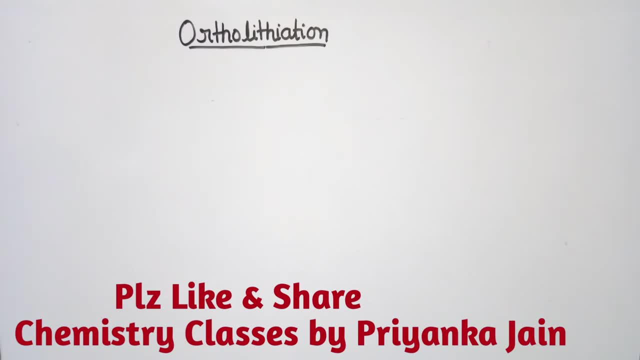 and here this will be the oh group. so this is the product. last, and the very important type of the reaction is the ortho lithiation reaction. what is it? it means the methylation at the ortho position to the substituent in the aromatic ring. so there should be a heteroatom. it means 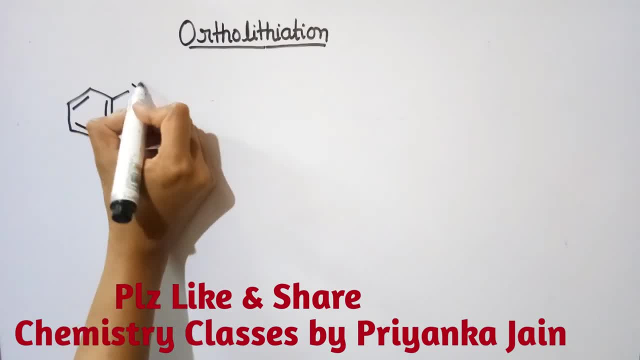 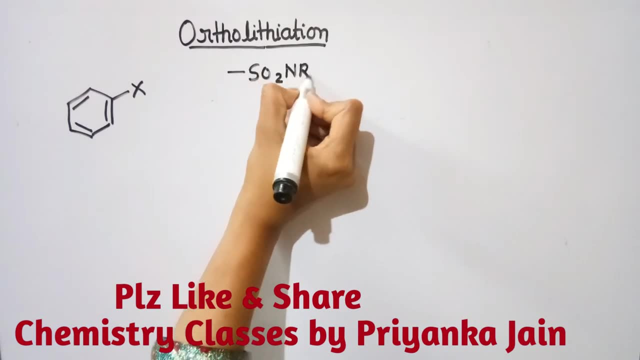 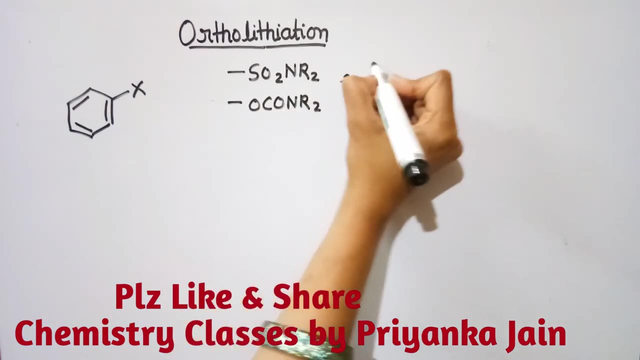 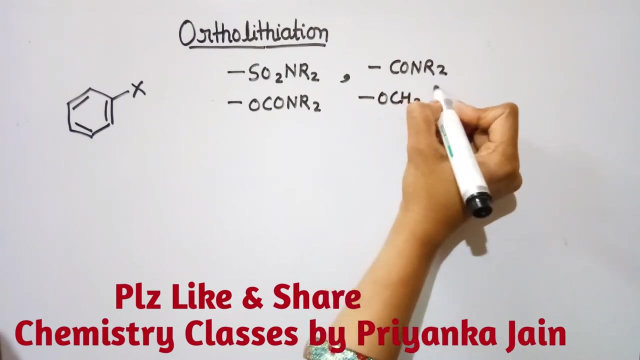 this ring should have a heteroatom present. this position: what is this heteroatom? this heteroatom may be either SO2NR2 group, or it may be OCONR2 group, or it may be CONR2 group or OCH2OME group. 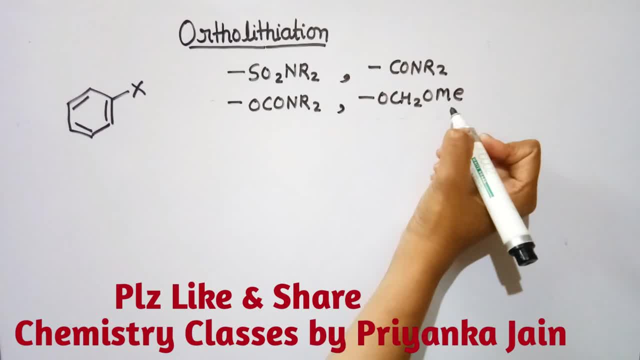 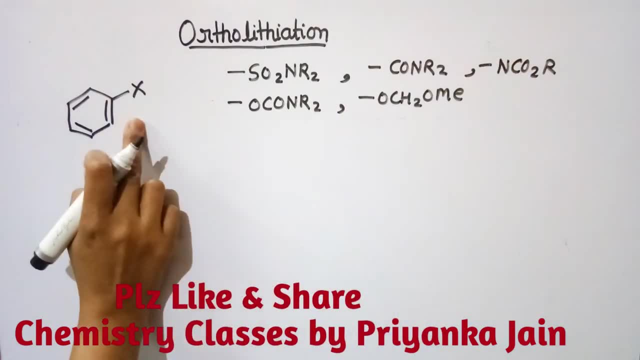 or it may be NCO2R group. such type of groups are, if present at this position in the aromatic ring, then if we treated with the N-butyl lithium or any of the organolithium present, then there will be a placement of the metal- it means lithium- at the ortho position to this. 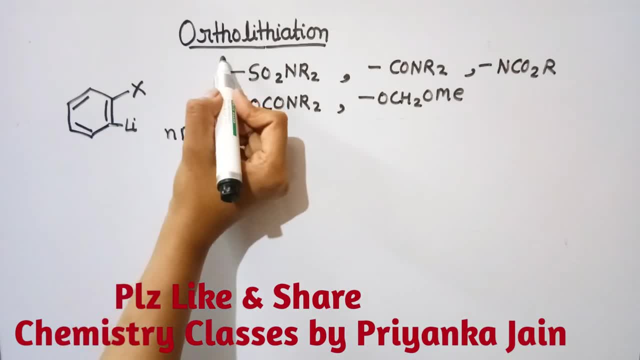 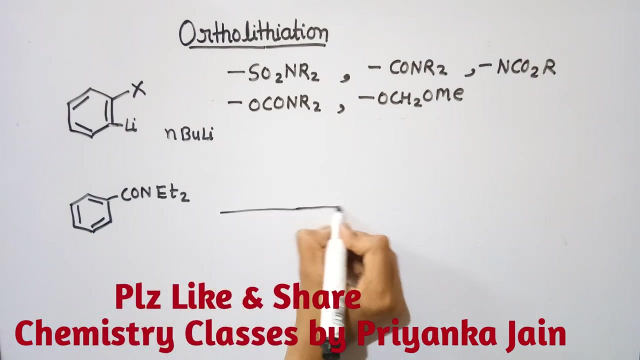 heteroatom. This is called the ortholithiation. I am taking here one example, simplest one, because unnecessary examples are not very important. We have to just clear the things. So this is the heteroatom that is present in this aromatic ring and if we are treating it with the 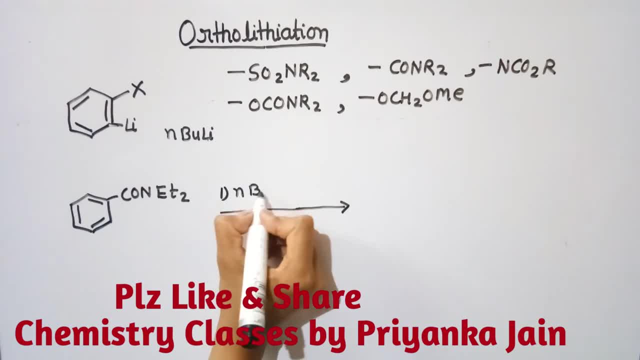 N-butylithium. sorry, we are treating it with the secondary butylithium in the THF at minus 78 degrees centigrade, and then we are treating it with the MEI- MEI. okay, So what will happen here In the first step, when we are treating it with this? 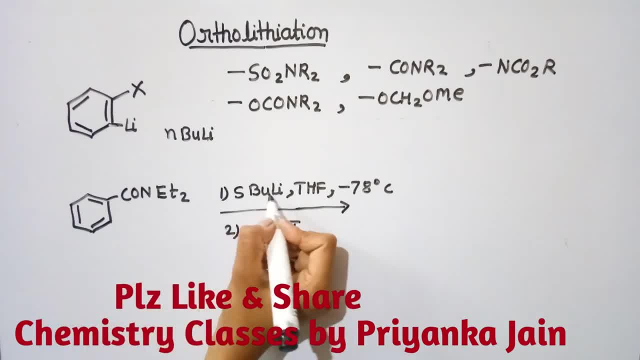 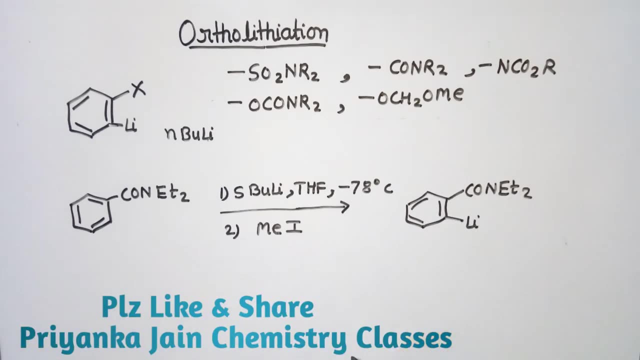 secondary butylithium. so here will be the placement, The placement of this lithium at this position: in the first step, This is CONET2, and here this is placed, and in the next step, when we are treating it with the MEI, then this lithium is replaced by this methyl group. So now here will be the methyl group. 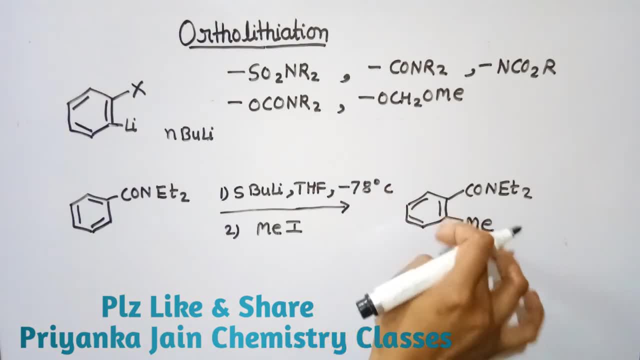 So in this way we can create a new group at the ortho position to this heteroatom By the reaction of ortho lithiation. So these are the some examples that are very important from the point of view of the NET and the GATT exam that I have taken here, and this is all about